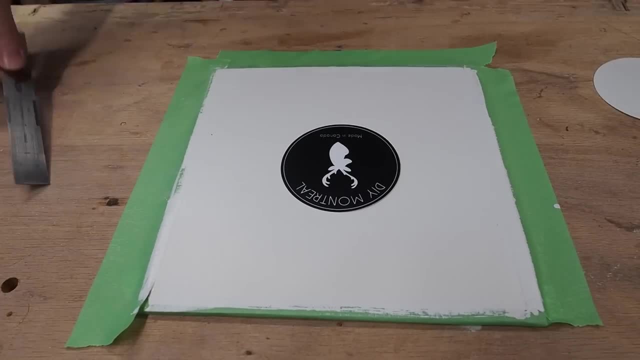 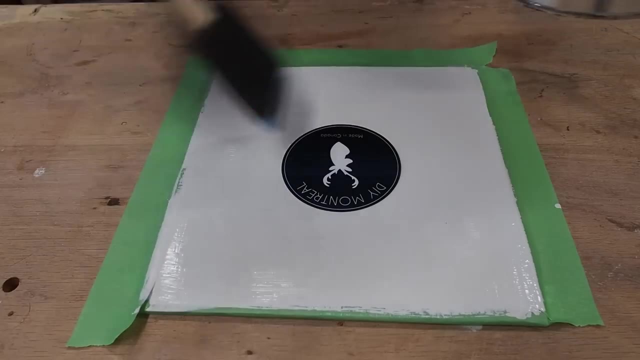 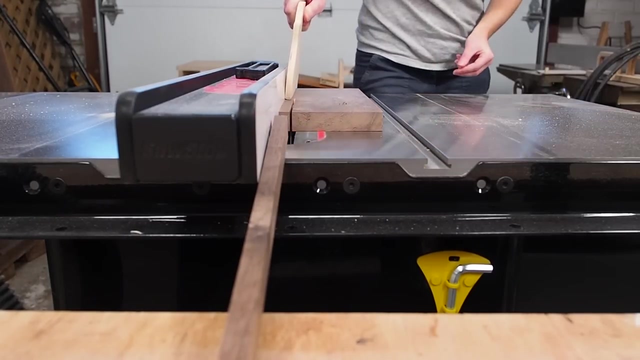 that I sealed with two coats of clear water-based poly. I used a Mosscast inksaw, which is much easier to use than the one on the standard one. While that was drying, I cut four thin strips of walnut Using a stop block on my miter saw. I cut the miters on all four pieces. 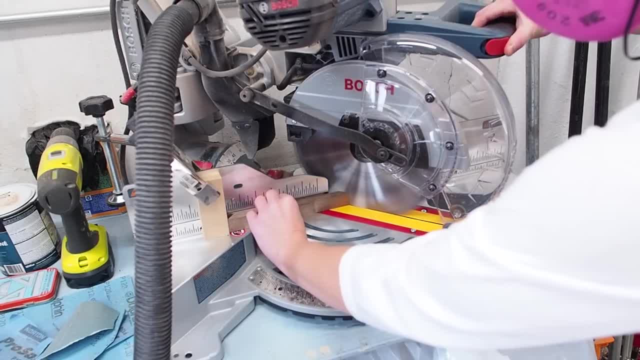 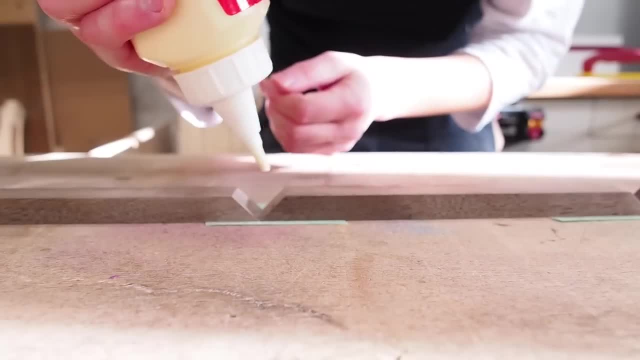 so that they would all be at the same length, And because this is so small, I was able to simply use some painters tape that I pre-applied, and I Then just folded it all up and sealed the last corner with some more tape, making sure. 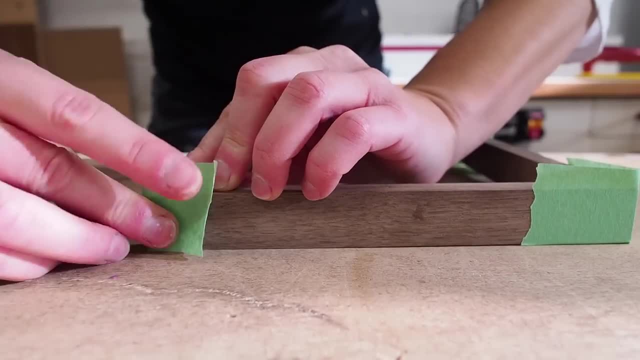 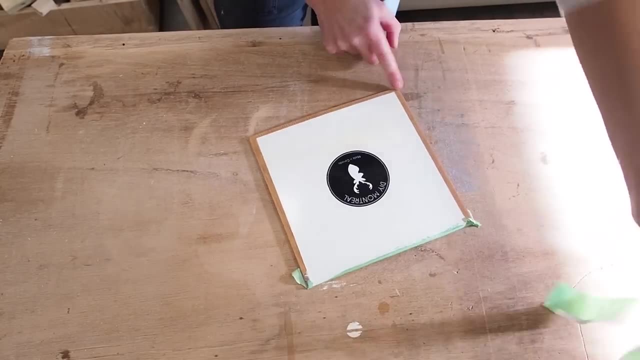 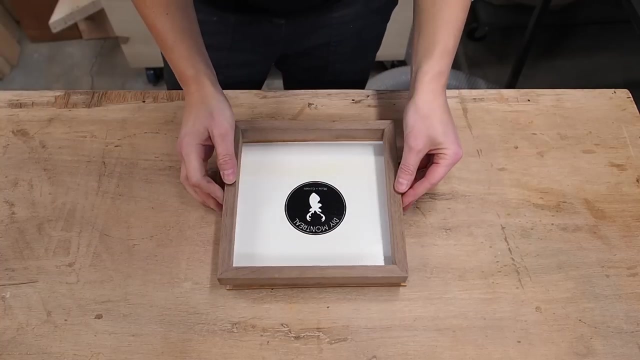 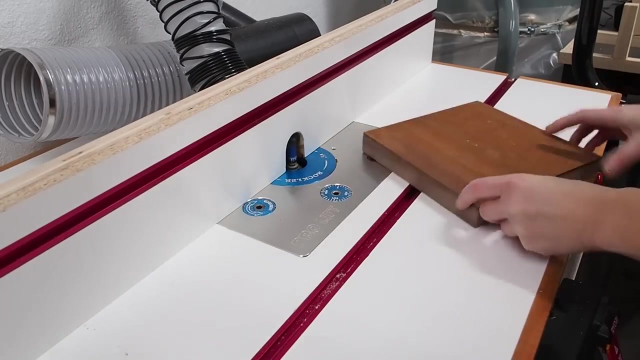 to wipe off all the excess glue while it was still wet. Ok, back to my backer board. I removed the tape and applied some glue to the frame and used some spring clamps to hold it while it dried. Lastly, I cleaned up the base on my router table by trimming the edges square with a 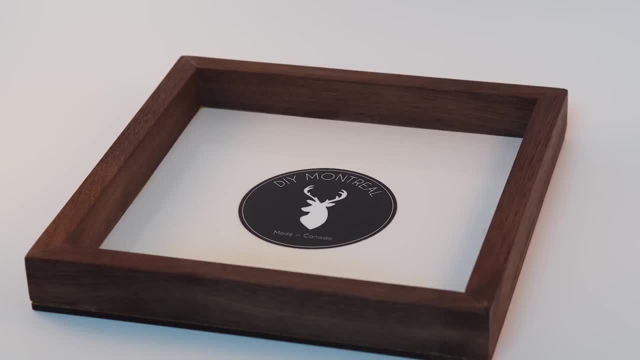 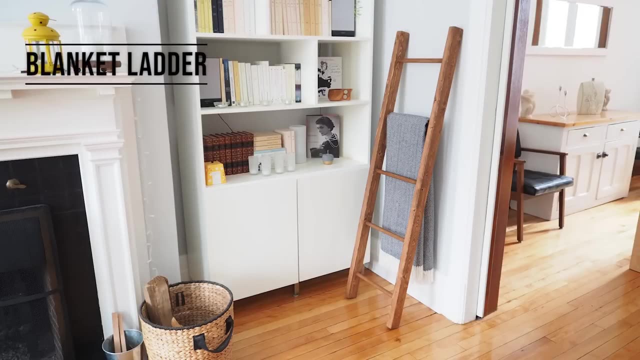 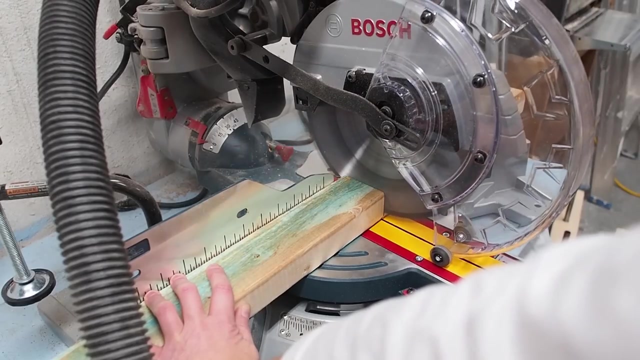 flush trim bit. Next up is a blanket ladder, and this is one of my favorites. All you need are two 2x3s and a couple dowels. I started by marking my 2x3 at 5 feet long, then cut them to length. 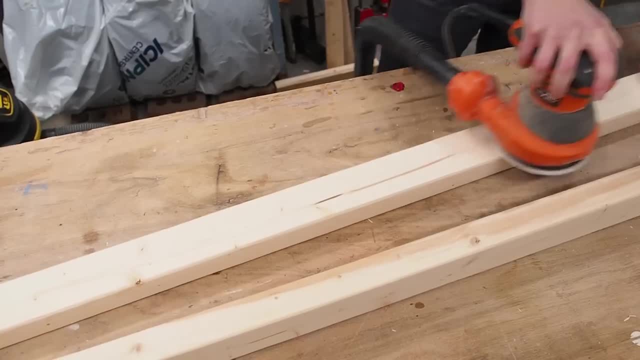 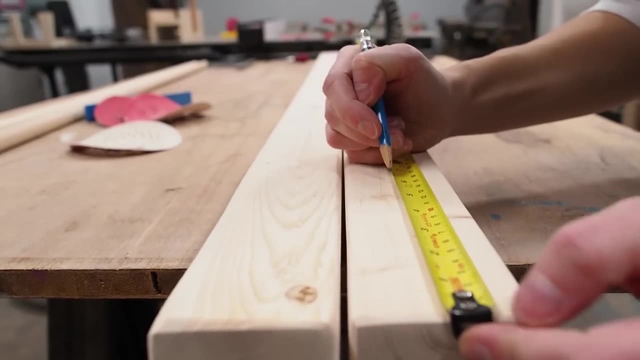 You'll notice, my lumber is bluish and pretty rough looking, so I spent a lot of time sanding from a low grit progressively up to a higher grit to make them nice and smooth. I'm going to add 5 ladder rungs, the first at 6 inches and then every 12 inches. 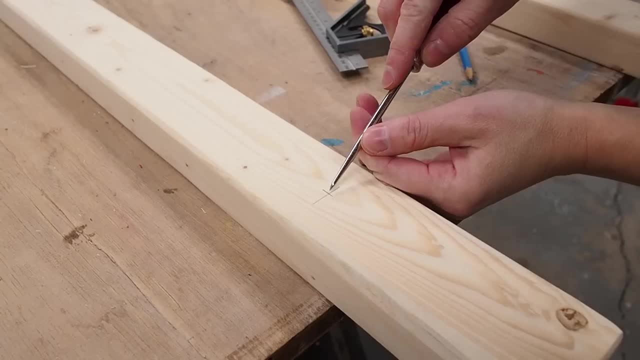 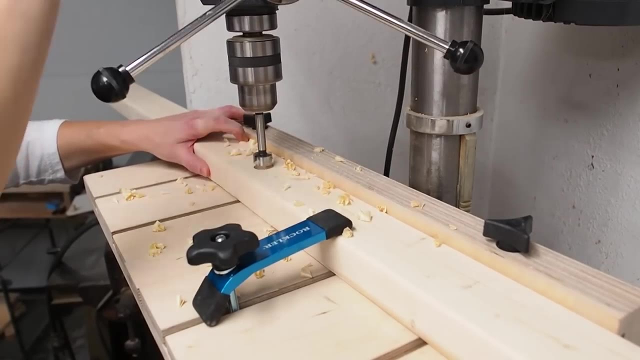 I found the center of the board and marked it with an awl. I then used a depth stop on my drill press to make sure that the holes were all at a consistent depth, and made the holes using a fastener bit that matches the size of the dowels that I'm 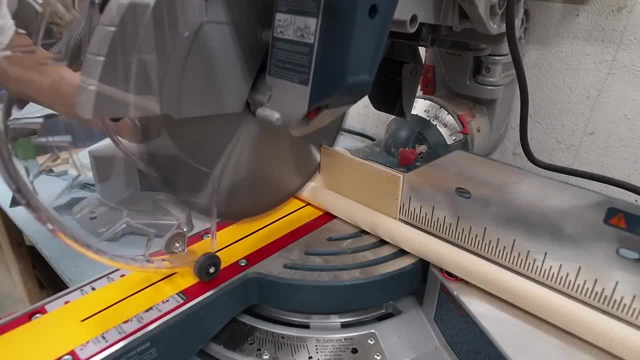 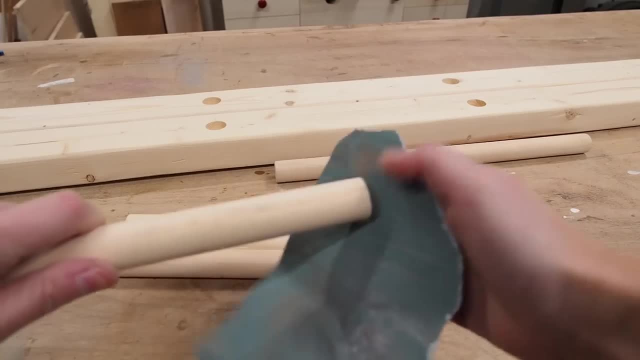 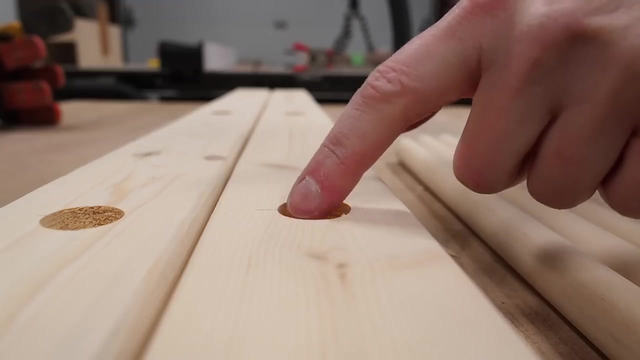 using, in my case, 7, 8's. Using a stop block, I cut 5 pieces of dowel at 14 inches long. It's a good idea to sand the ends a little to ease the fit, And the glue up is super simple if you start with one side, then fit it into the other. 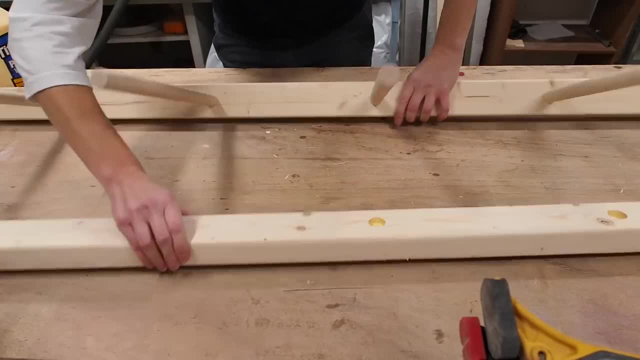 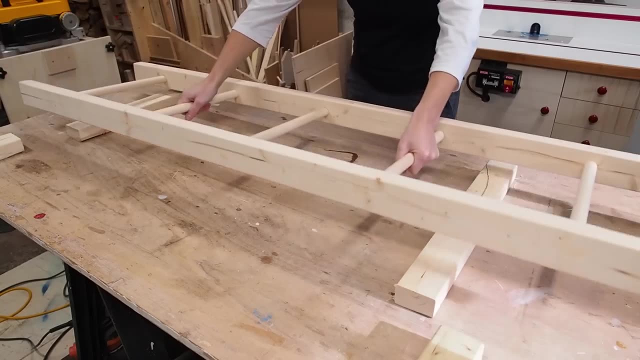 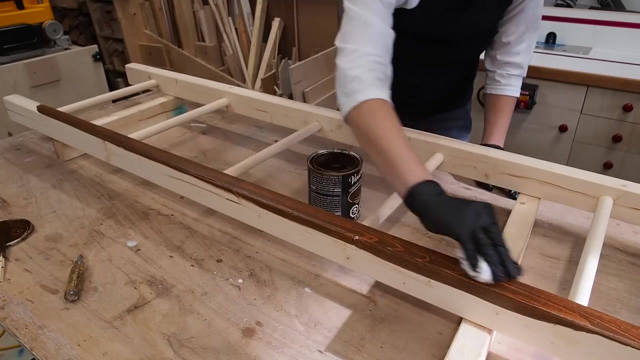 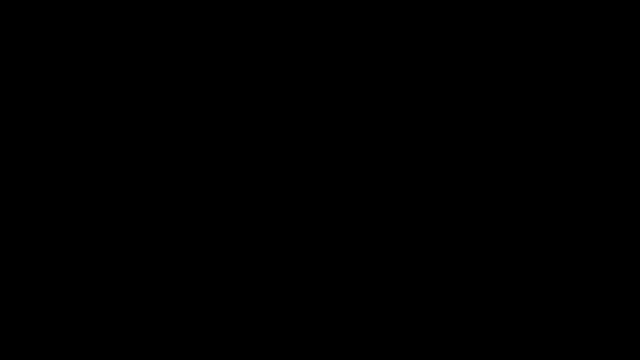 side. Just make sure to have all your clamps ready. And there you have it. I hope you enjoyed this video. I'll see you next time. Bye, Bye, Bye, Bye, Bye. To finish off, I applied some stain and used a wipe-on poly as a finish coat. 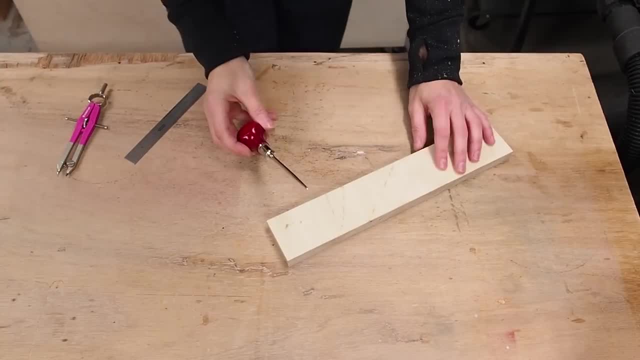 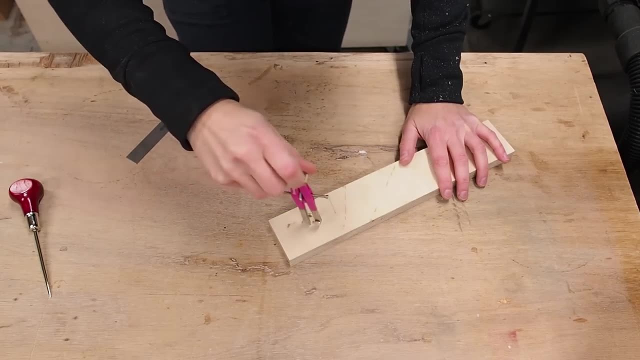 Next up is a simple yet elegant plywood ring. For this I'm using 3.25 inch baltic birch plywood. I started my punching a small hole using a scratch awl, Using that as the center point. I used a compass to trace all the holes. 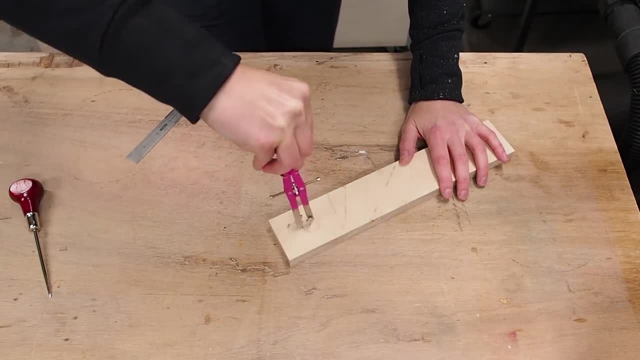 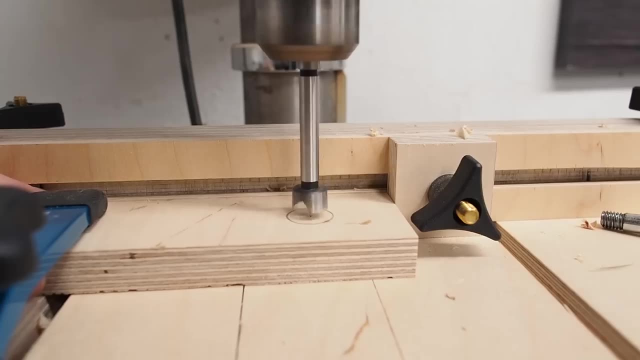 Then I permed it by: assemble it like you make on my board, used a compass to trace a circle. Then, over at the drill press, I started by punching a hole all the way through the center using a small bit. This will show me where the exact center is, so I can drill halfway with a forstner bit. then 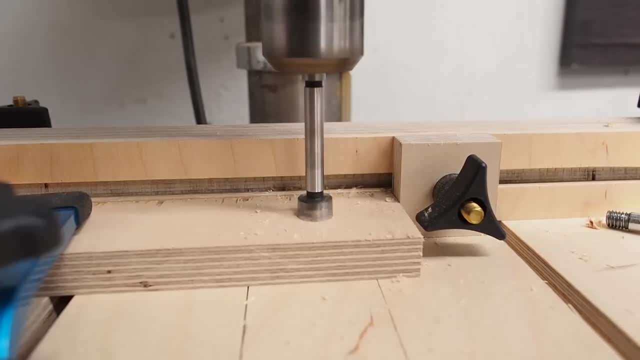 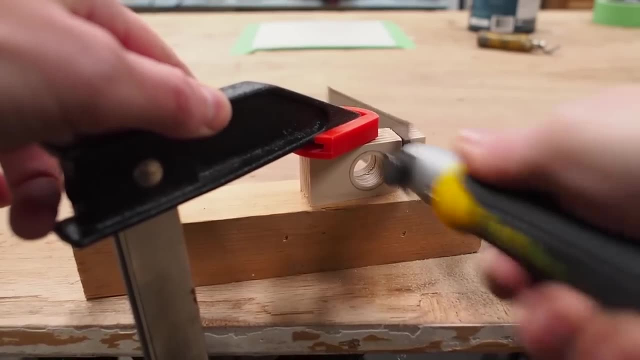 flip it over and finish from the other side, avoiding any potential tear up To shape the ring. I started by cutting down the block as close to the line as I could get, before taking it over to my sander and sanding it right up to the. 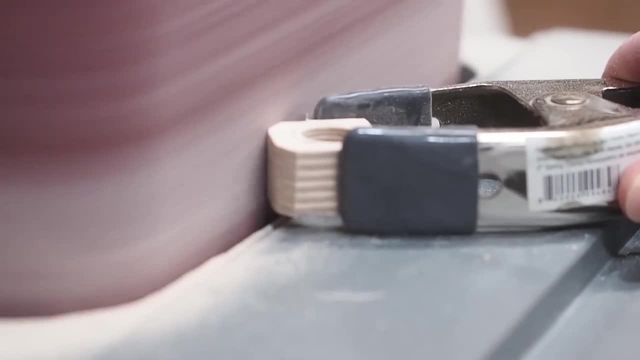 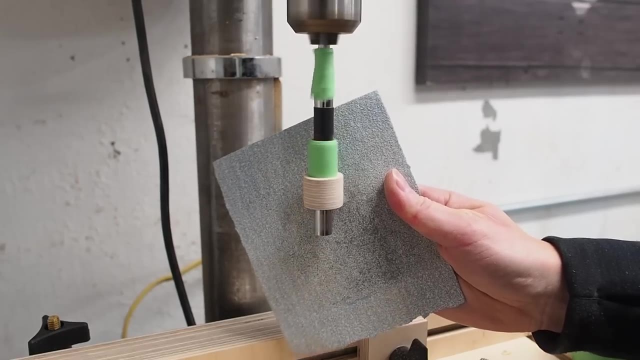 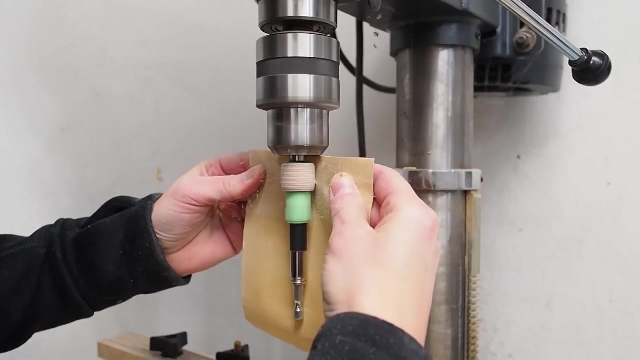 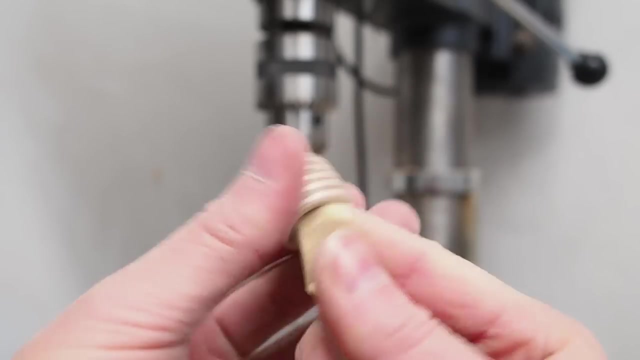 line all around. After that I used some tape so I could hold the ring on a bit and use my drill press to help me sand the ring all around. I progressively moved to finer grit paper and made sure to round the outer edges as I went To. 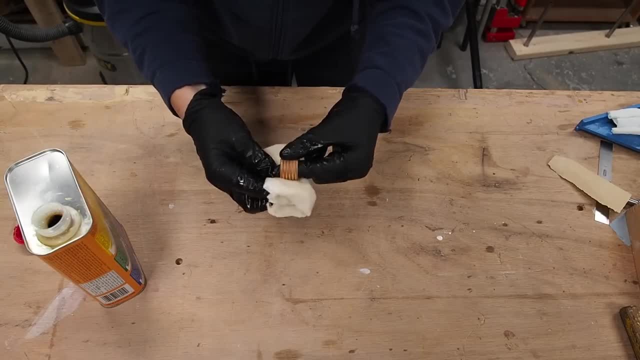 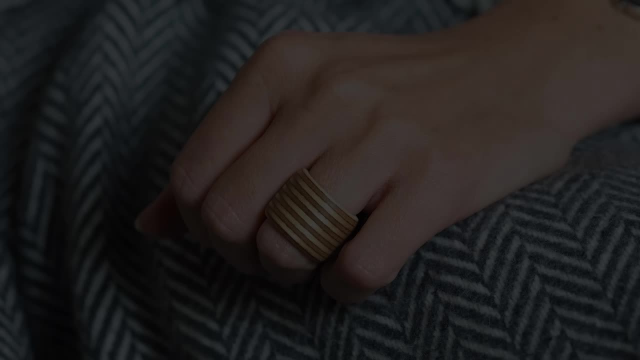 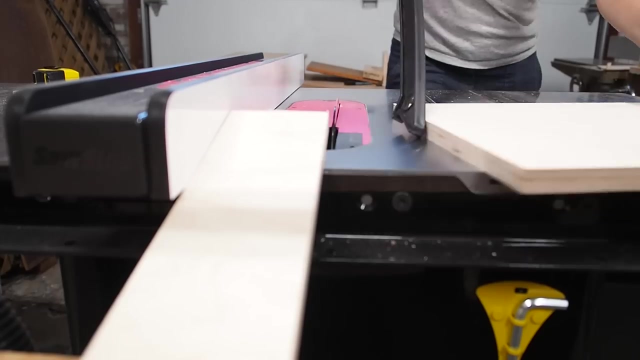 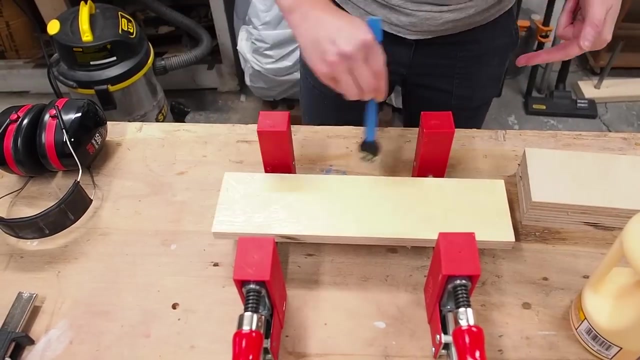 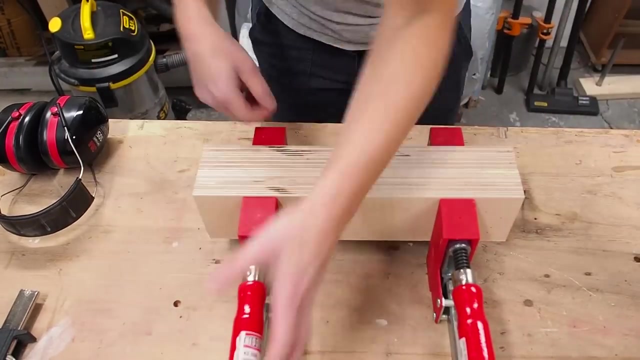 finish off, I applied several coats of tongue oil. I I, I Alright. next up is a plywood pencil holder. For this I'm again using Baltic birch plywood because I love the look of the crosscut. I cut four equal pieces and made a sandwich by gluing them all together. After the block is finished, I 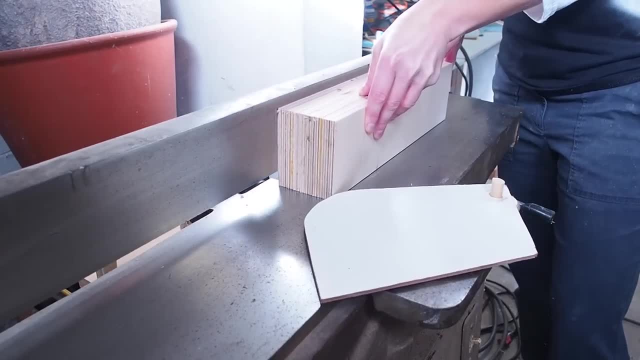 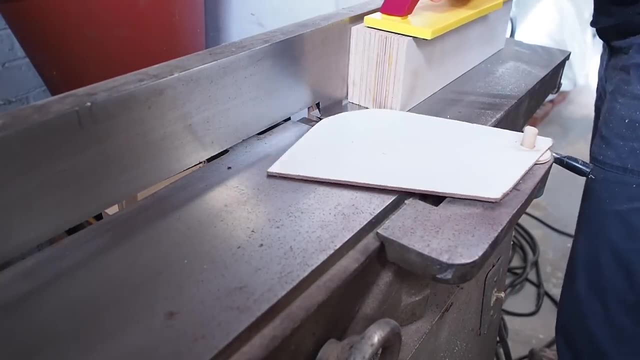 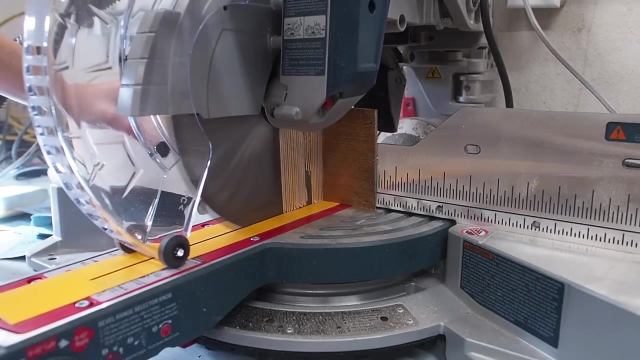 I used a chisel to clean off some of the dry glue before running it through my jointer to square up the faces, And I did this on both sides. You could just as well use a planer. I then squared off the end using my miter saw and made a first. 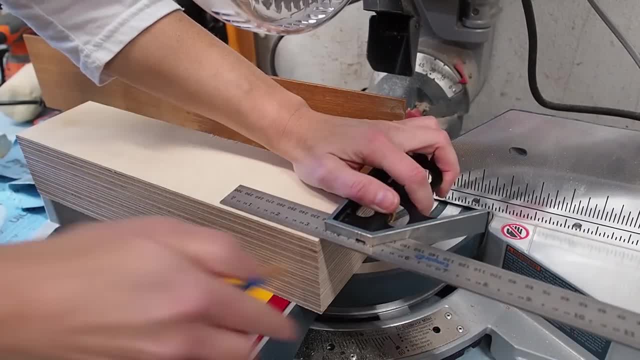 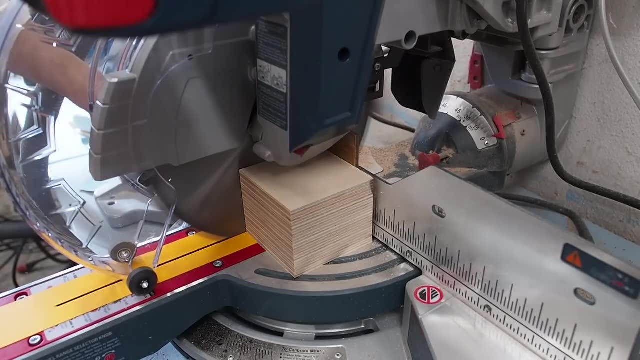 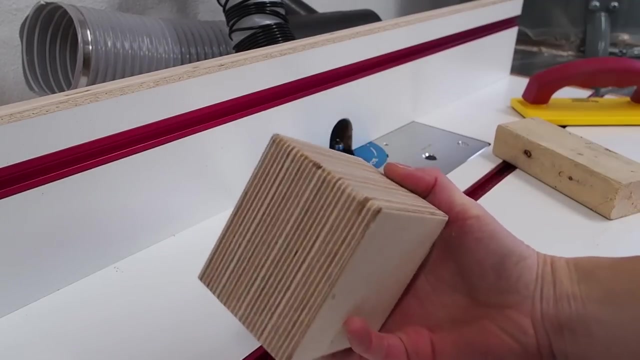 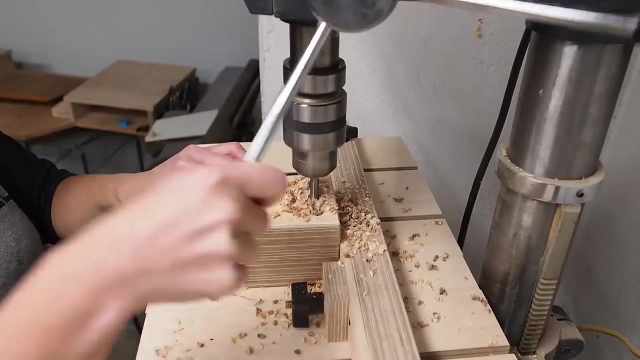 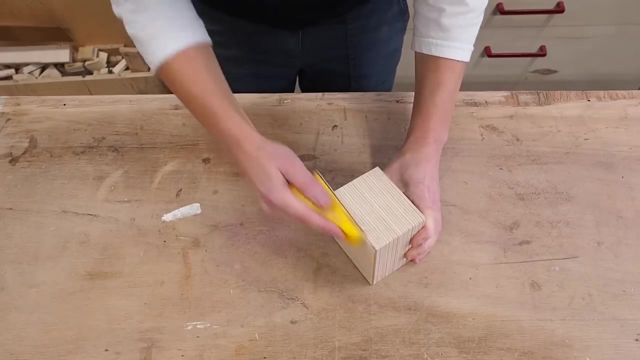 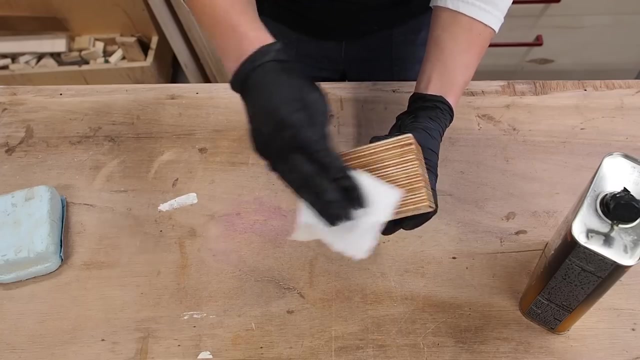 cut of a block that was nice and square. I, I, I- I effectively cut a piece of plywood around the top edge, so I need to do a little bit of sanding. I stuck the two pieces together at the back so I can put one in at each end and not get all the reinforcing bolts in the face. I could just put them all in. 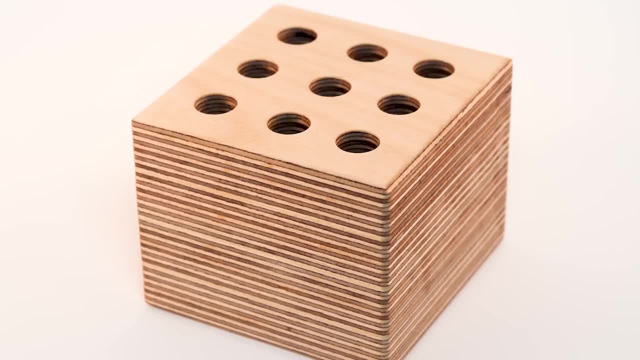 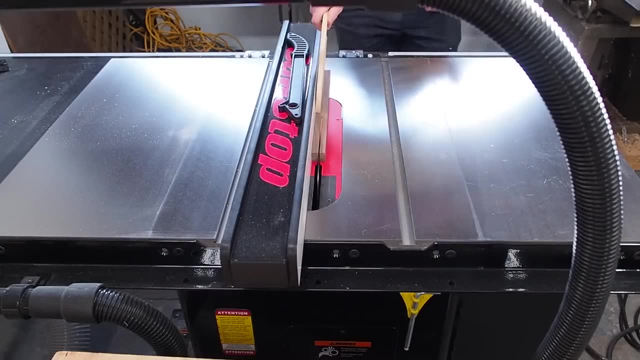 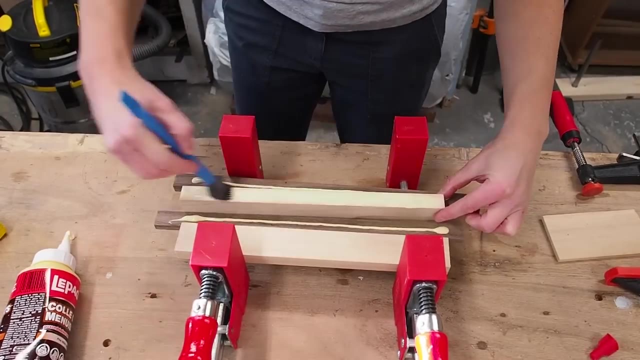 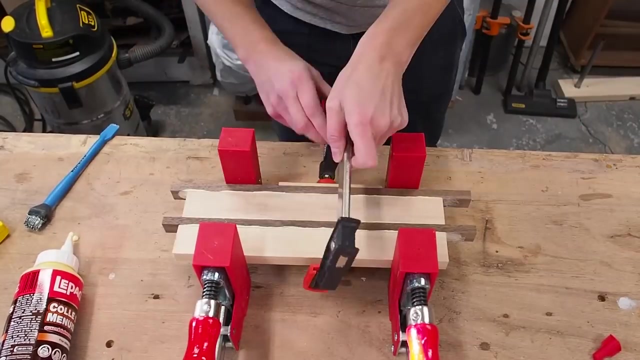 Another simple project that you can customize is a business card holder. I started by cutting up a few scraps and arranged them into a pattern that I liked. After a quick glue up, I ran it through the planner a few times, on both sides, to even. 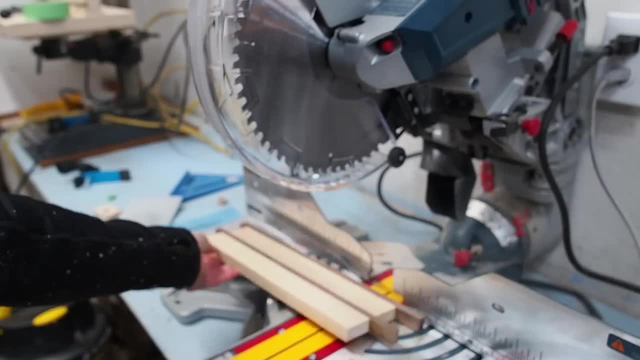 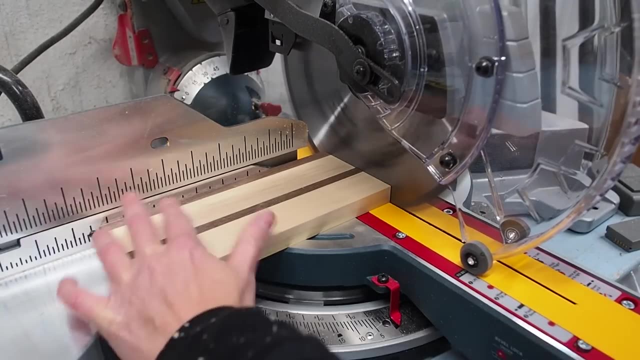 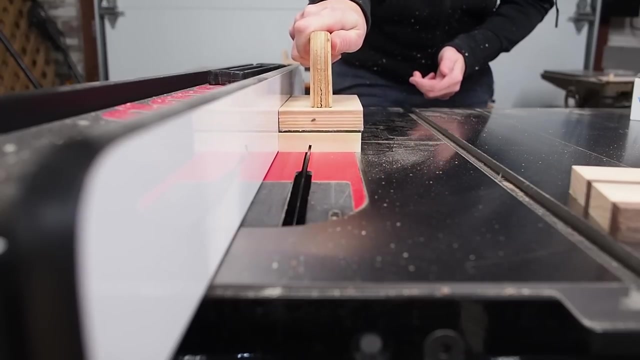 it out. I then squared the ends and cut a few randomly sized blocks Over at the table saw I tilted the blade just slightly, maybe 5 or 10 degrees. I then ran the block through several times, slightly adjusting my fence at each pass. 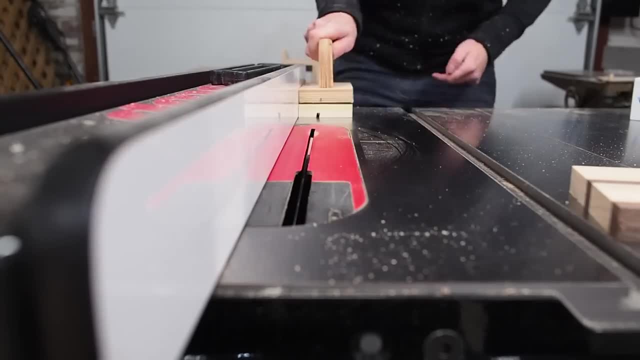 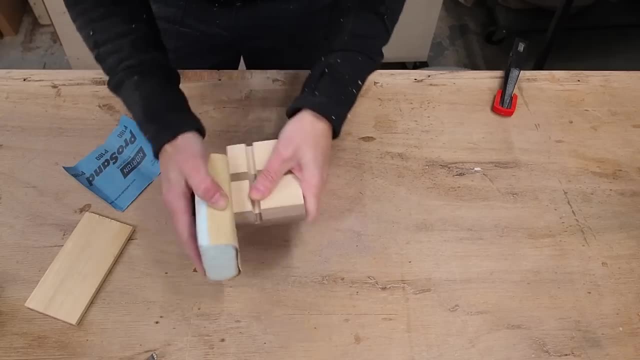 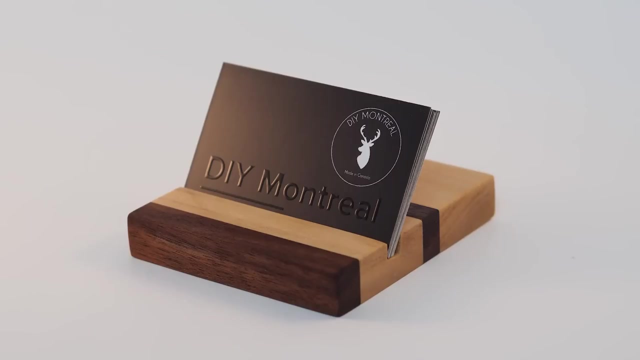 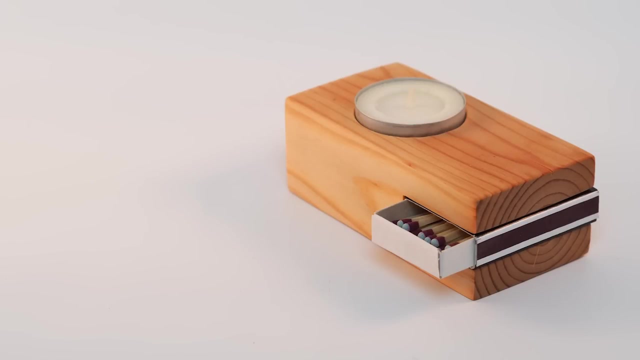 in order to make a thin shallow groove. And there we go. After some sanding, I finished off these as well with a few coats of tongue oil. That's all there is to it. Hey, I hope you enjoyed this video and I hope it sparked some ideas for gifts that you could. 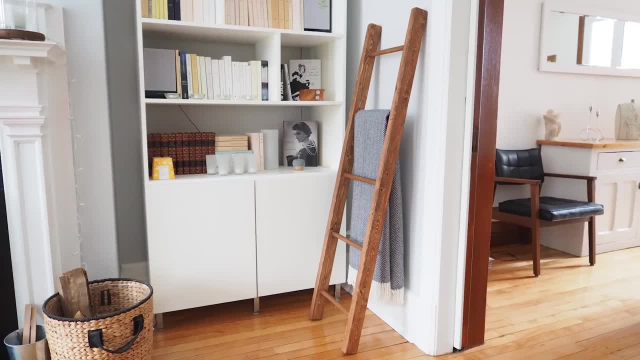 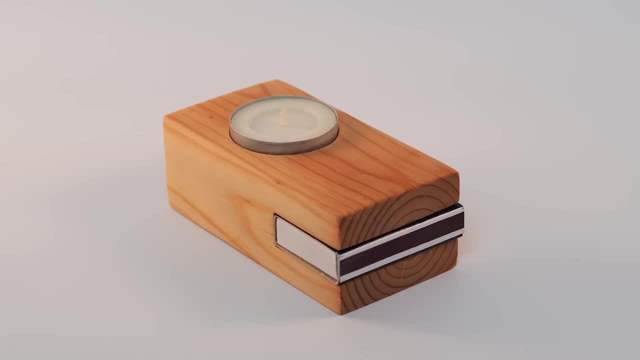 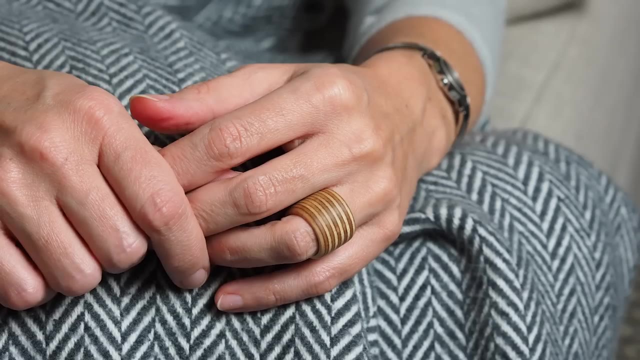 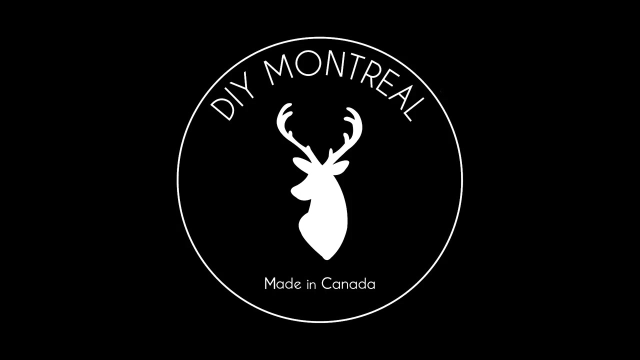 make yourself. Stay tuned for a few more ideas coming up from my previous videos, and if you have any other ideas, be sure to leave those in the comments below. Until next time. thanks for watching. I'll see you in the next video. bye.